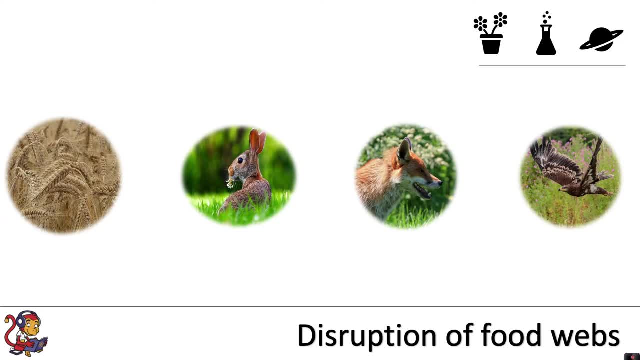 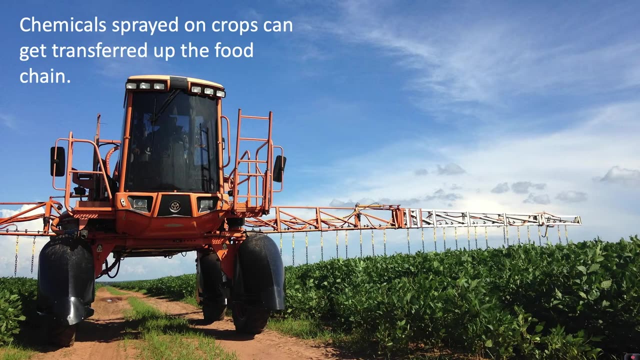 going to do that by looking at a particular food chain where we've got the wheat and then the rabbit and the fox and the eagle, And we're going to look at how chemicals can be passed along a food chain, So chemicals are sprayed on crops and they get transferred. 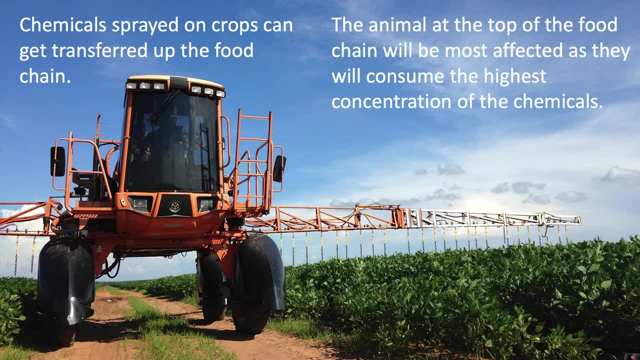 up the food chain. The animal at the top of the food chain will be most affected, as they will consume the highest concentration of the chemicals. This is called bioaccumulation, because bio means living things and accumulation means building up, So it's the idea that these chemicals build up in these living organisms. So a farmer 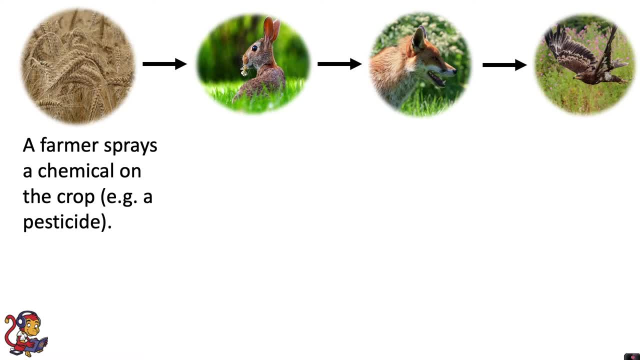 sprays a chemical on the crop, for example a pesticide, and the rabbit will eat the crop and the chemicals will build up in the rabbit. The fox will eat many rabbits And we'll have the chemicals from all of the rabbits building up inside it. 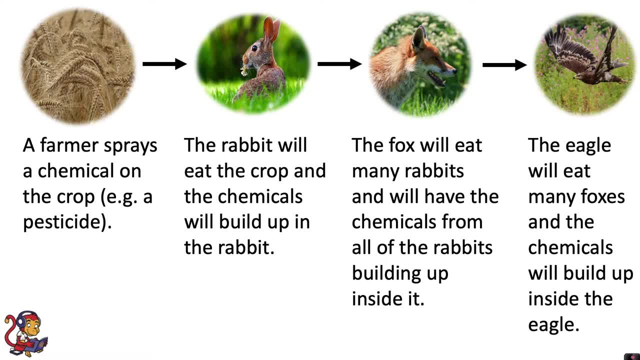 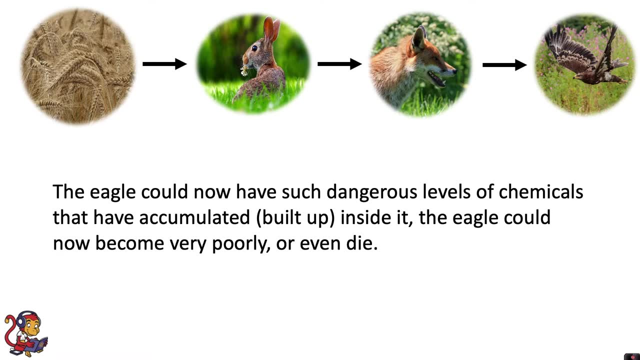 And the eagle will eat many foxes And the chemicals will build up inside the eagle And, as we said, the eagle will have the highest concentration of chemicals built up inside it. So the eagle could now have such dangerous levels of chemicals that have accumulated. 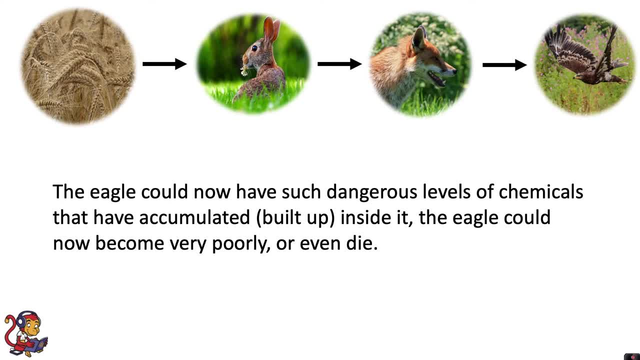 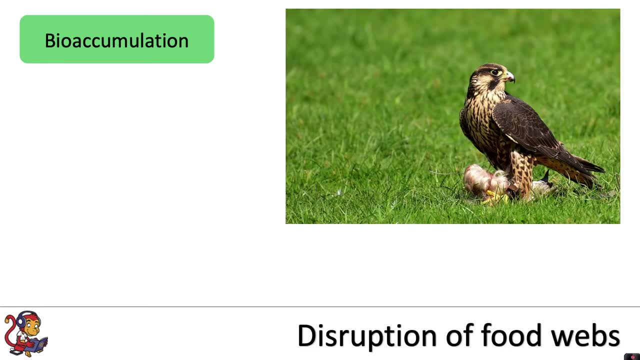 which means built up inside it, The eagle could now become very poorly or even die. Now we're going to look at a case study of bioaccumulation with a chemical called DDT. DDT was an insecticide used to kill mosquitoes. This was used widely to help against the spread. 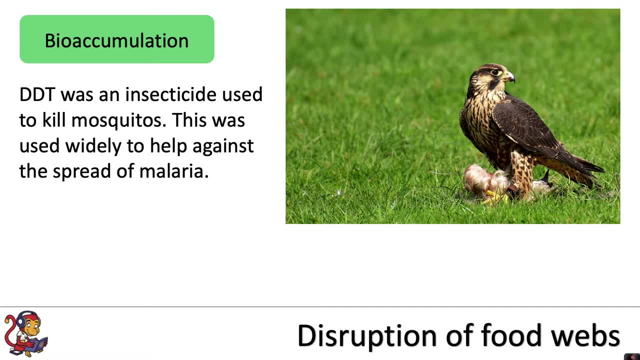 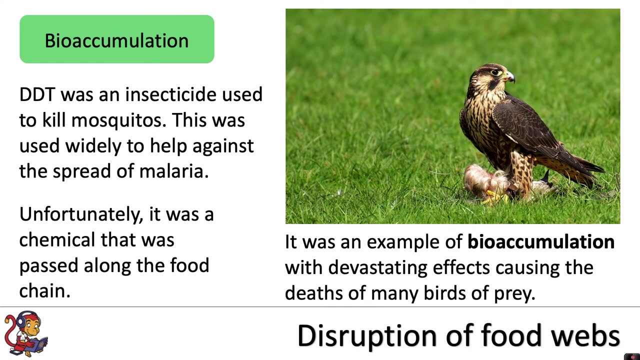 of malaria, and it was also widely used as an insecticide on crop fields. Unfortunately, it was a chemical that was passed along the food chain. It was an example of bioaccumulation with devastating effects, causing the deaths of many birds of prey. 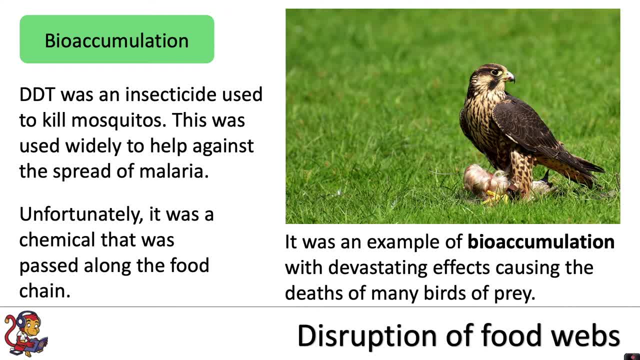 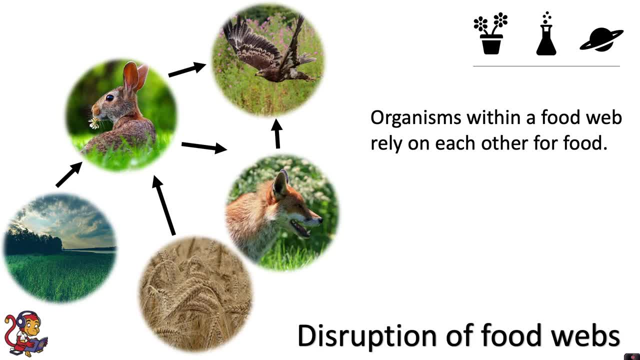 This, of course, will have a knock-on effect to the whole of the food chain or, more widely, the whole of the food web, Because organisms within a food web rely on each other for food. This is an example of interdependence. And if one of those animals were to be wiped out, as we said, through perhaps disease or